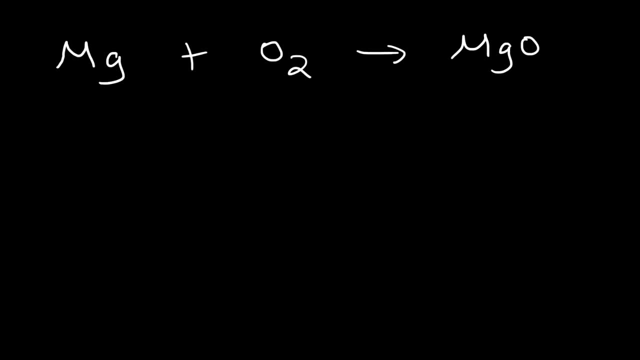 Now, perhaps you found or watched my video on oxidation numbers. If you have, then you know that the oxidation number of any pure element is zero. Now, in magnesium oxide, magnesium, being an alkaline earth metal, has a charge of plus 2.. Oxygen has a charge of minus 2.. Notice that the oxidation state of 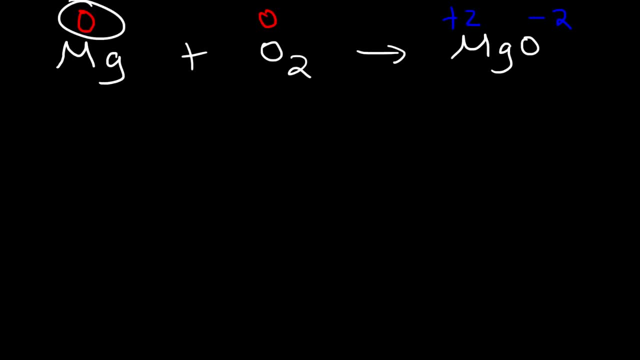 magnesium went from 0 to plus 2. So the oxidation state increased. Whenever the oxidation state goes up, the substance is said to be oxidized, And if you take a look at this video, you'll notice that in the case of oxygen, the 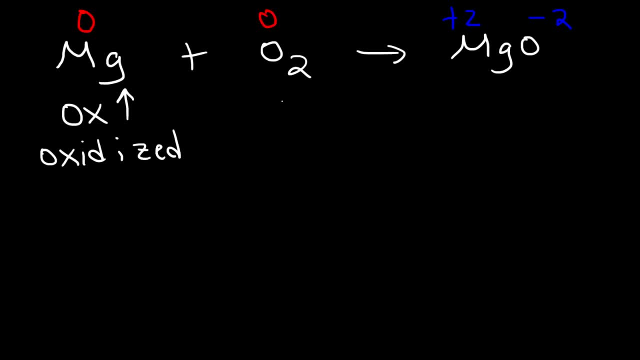 oxidation number decreased from 0 to negative 2.. Whenever the oxidation number decreases, the substance is being reduced. Now you need to know that oxidation always occurs with a loss of electrons. Reduction is associated with a gain of electrons. Metals: they like to give away electrons. 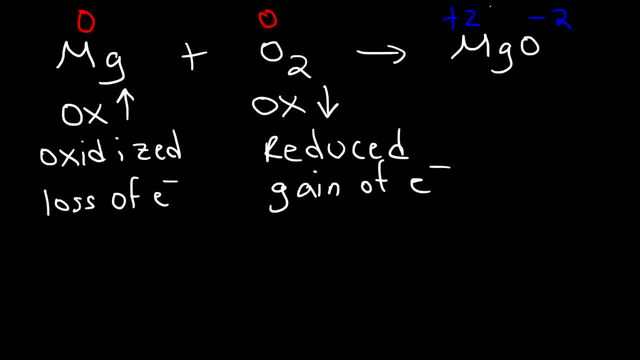 Metal cations, As they give away electrons, they will acquire a positive charge. Non-metals, like oxygen, they like to acquire electrons, and so they will develop a negative charge. The substance that is oxidized is known as the reducing agent, And the substance that is reduced is known as the oxidizing agent: Metals. 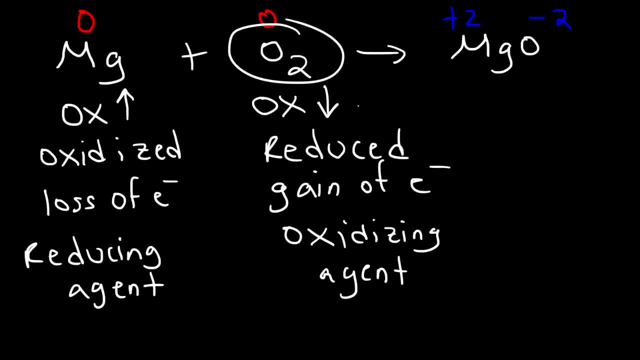 are reducing agents because they are oxidizing. They are oxidizing because they are causing the other substance to be reduced. Non-metals, like oxygen, gas, fluorine. they're oxidizing agents because they cause another substance to be oxidized. And that's where you got to see it. So these are some terms that you 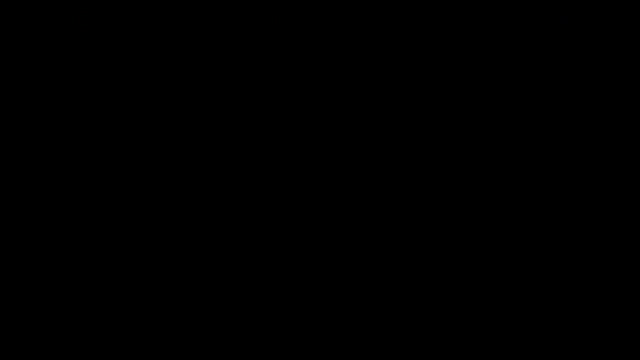 want to be familiar with when dealing with redox reactions. Now let's go back to that reaction, The reaction between magnesium and oxygen gas. Now magnesium, it's changing into the magnesium ion. This magnesium ion has a plus two charge And in order to become a plus two cation it has to lose two electrons. Now oxygen. 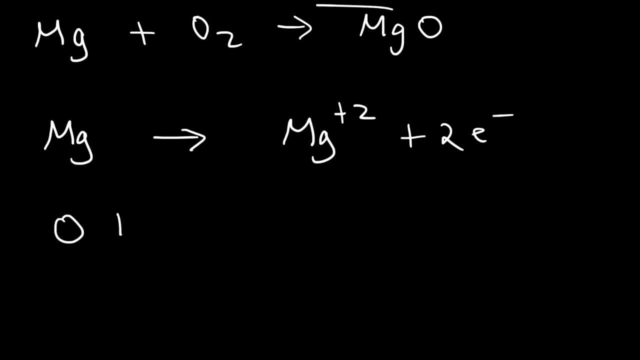 I'm going to write atomic oxygen because this reaction is not balanced. Individually, oxygen acquires two electrons and turns into oxide. Now, because magnesium lost electrons, this reaction, which is known as a half reaction, that's, the oxidation part of the reaction- 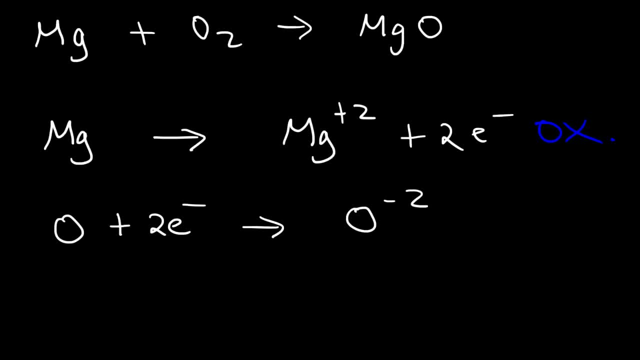 Anytime a substance loses electrons, it's being oxidized. This second half reaction is the reduction part, since oxygen is acquiring electrons. Whenever a substance gains electrons or if the oxidation number decreases, it's reduction. Now for half reactions. anytime you have electrons on the right side, it's going to be an oxidation half reaction. Whenever 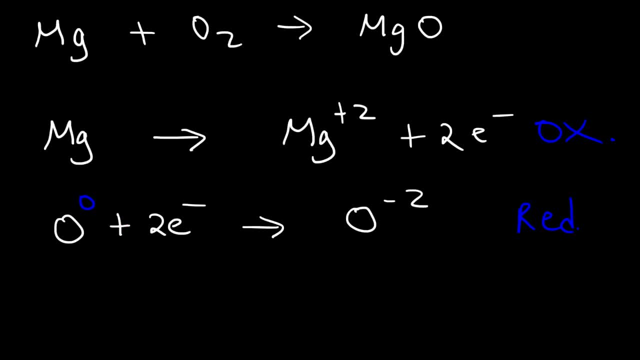 the electrons are on the left side. it's a reduction half reaction. That's another way in which you can see it too. Consider this reaction: Zinc metal reacts with hydrochloric acid to produce hydrogen gas and zinc chloride. Identify the substance that is oxidized and 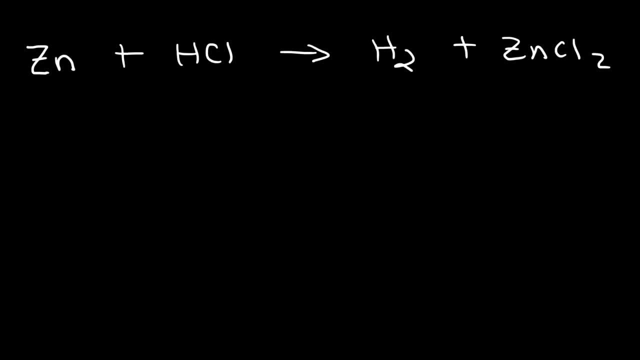 the substance that is reduced And also identify the oxidizing agent and the reducing agent. Now, if you get a question like this on the test to find a substance that is oxidized or reduced, always look at the reactants. It's one of these two. Don't look at the products. 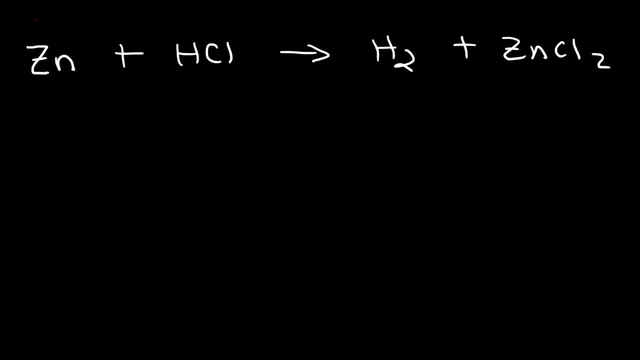 Now let's find the oxidation states of everything. The oxidation state of any pure element is always zero. Now, whenever hydrogen is bonded to a nonmetal, it's going to have a positive one oxidation state, which means chlorine has to be minus one. 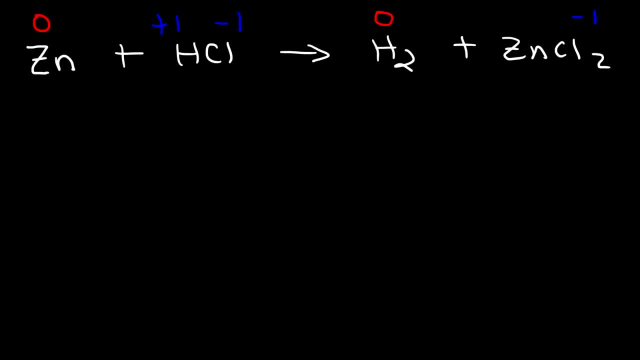 Now, in this one too, chlorine is still negative one, which means zinc has to have a plus two charge. Now the oxidation of zinc changes from zero to positive two, So zinc is being oxidized. Hydrogen changes from one to zero, So HCl as a substance is being reduced even. 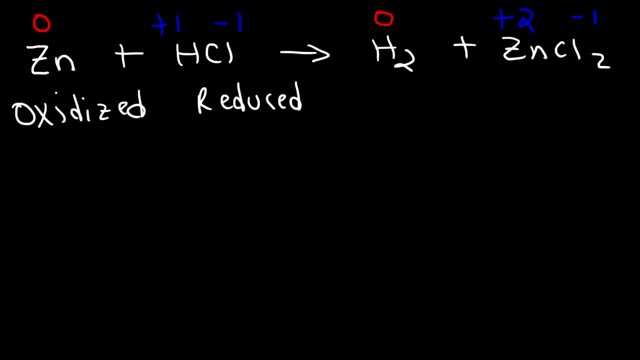 though only the hydrogen portion of that substance is being reduced. So typically if they ask you for the substance, even though it's only the hydrogen element that's being reduced, you would say the whole substance is being reduced. if you have to choose an answer on a multiple choice test, 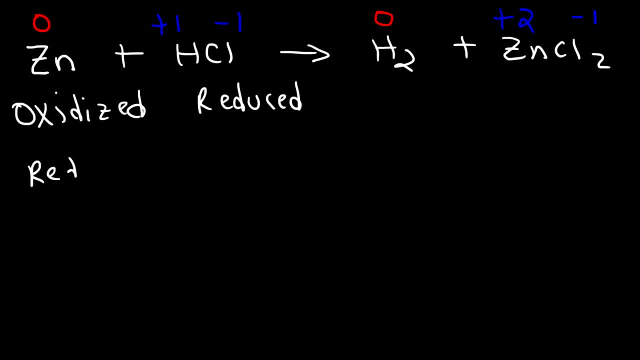 Now, the substance that is oxidized is the reducing agent, And typically metals tend to be reducing agents. The substance that is reduced is the oxidizing agent, And this is a common question that you might see on a typical chemistry exam. Now let's try one more example for the sake of practice. Methane reacts with oxygen gas. 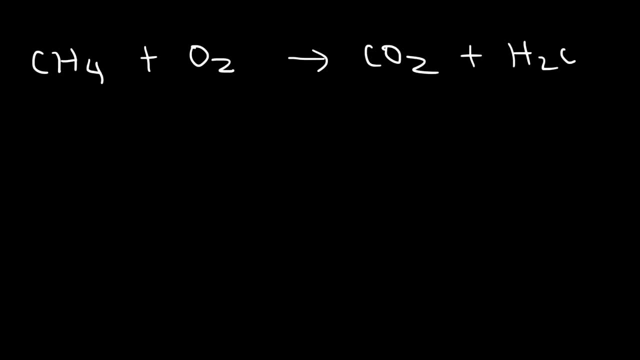 and it produces carbon dioxide and water. So feel free to pause the video, identify the oxidation states of every element in this reaction and then find the substance that is oxidized, reduce and identify the oxidizing agent and the reducing agent. So let's identify the pure elements, which is only oxygen gas. That's going to be zero. 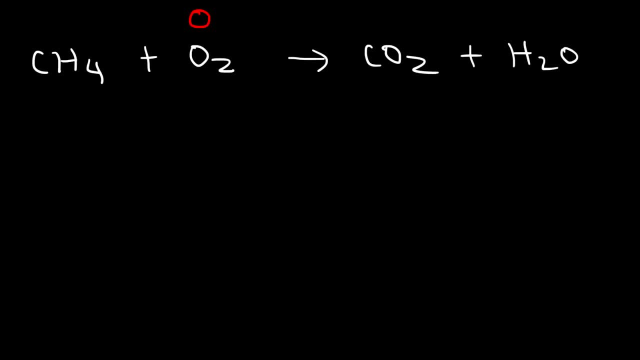 Now we said that whenever hydrogen is bonded to a non-metal, it's going to have a plus one oxidation state, And typically when oxygen is found in a compound, the oxidation state is negative two, except when it's bonded to fluorine or except when it's in the form of peroxide or superoxide. 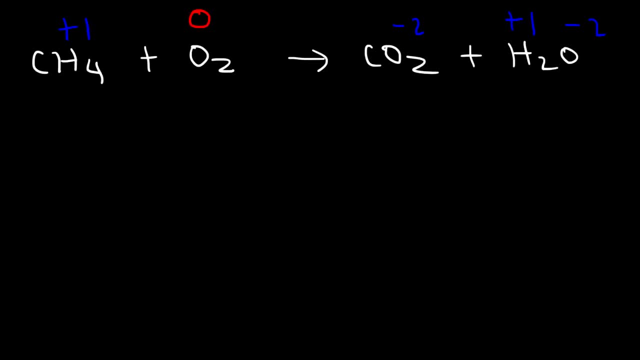 It's different. Whenever you hear the word oxide, the oxidation state of oxygen is negative two. If you hear the word peroxide, it's negative one. If you hear the word superoxide, it's negative one half. Now we've got to find the oxidation state of carbon, So let's start with methane. 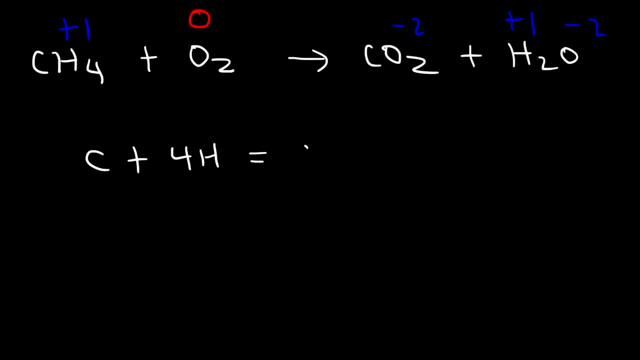 So we have one carbon atom and four hydrogen atoms, which has to add up to zero because methane is neutral in charge. Now each hydrogen atom has an oxidation state of one, So therefore C plus four must equal zero. Therefore, carbon has to have an oxidation. 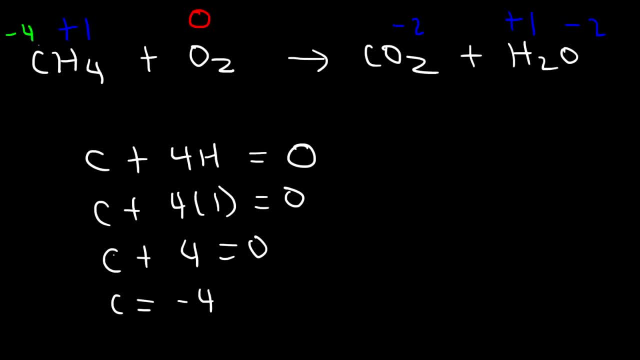 state of negative two. Now let's calculate the oxidation state of carbon in CO2.. So it's C plus two oxygen atoms, which equals a net charge of zero, And each oxygen has a charge of negative two. So in this case carbon is going to have an oxidation state of positive four. So carbon changes from negative four to positive four. Therefore the oxidation number of carbon is increasing, which means carbon is oxidized or technically, methane is oxidized. Now, hydrogen doesn't change, But oxygen changes from zero to negative two, So therefore oxygen gas. 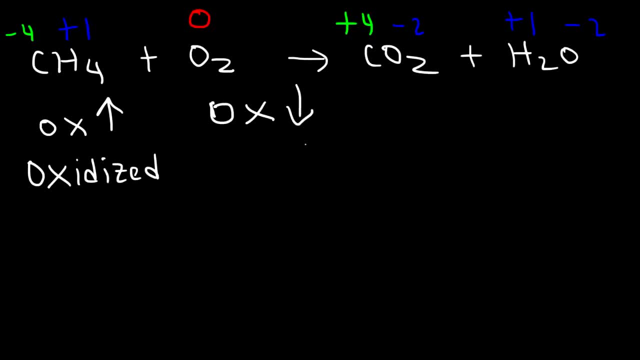 The oxidation number of CO2 is going to be negative two, So that means carbon is oxidized. The oxidation number is decreasing, So it's being reduced, Which means that methane is the reducing agent And oxygen gas it's being reduced, which makes it the oxidizing agent. 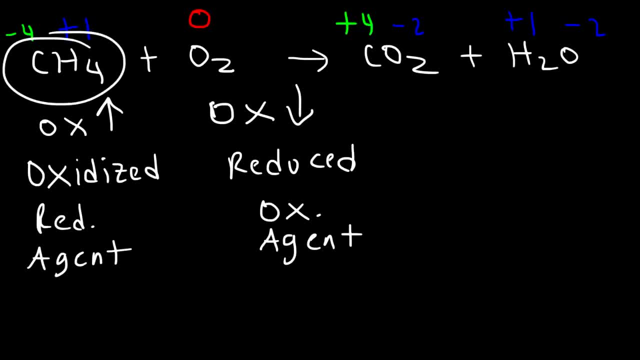 So, keep in mind, even though the element carbon is being oxidized, you would still describe the whole substance, methane, as being oxidized, because carbon is part of methane. Now, the next thing that you need to be able to do is you need to take a look at a reaction. 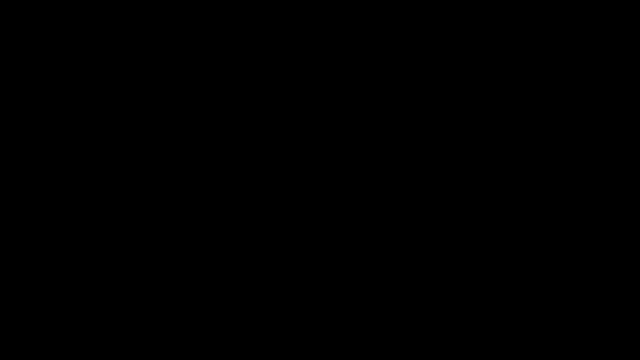 And tell if it's an oxidation reduction reaction. So consider this reaction: Aluminum metal reacts with copper chloride to produce aluminum chloride and copper metal. Is this reaction a redox reaction? So this reaction is a single replacement reaction And if there's a transfer of electrons then it's going to be a redox reaction. 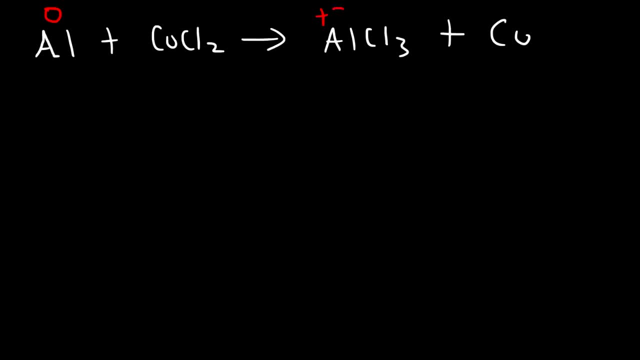 Aluminum has an oxidation state of zero, But in AlCl3, it has an oxidation state of plus three. So if the oxidation number changes, then it's a redox reaction. All single replacement reactions are redox reactions. Now, if you don't want to look for the oxidation numbers, there's a quick way to tell if something 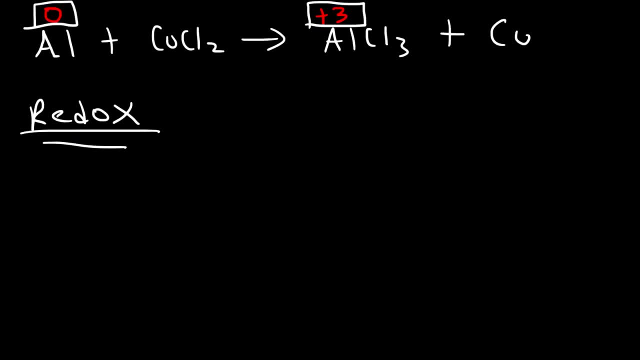 is going to be a redox reaction. If you see a pure element on one side and then that element being part of a compound on the other side, It's always a redox reaction. It's going to be a redox reaction. 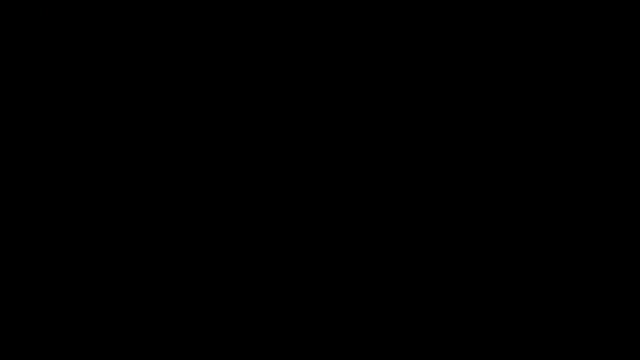 There's a transfer of electrons. So let me give you two examples And I want you to determine if it's a redox reaction or not. So both of these examples are synthesis reactions, also known as combination reactions. Sometimes a combination reaction can be a redox reaction. 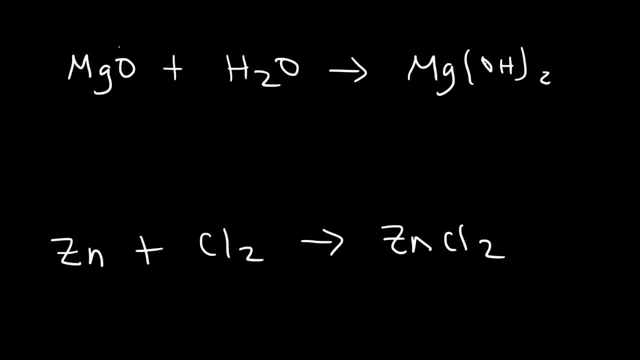 And sometimes it won't be. Now, if you look at the first example, there are no pure elements. All we have is compounds, When you see that chances are it's not a redox reaction. But if you look at the second example, we have a pure element, zinc, and then that same. 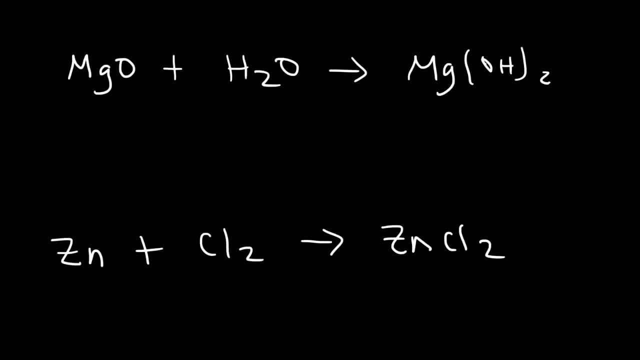 element is in a compound. So the second example is a redox reaction, And let's prove it. So let's start with the first example. Oxygen has a negative two charge. Magnesium has a negative two charge. Magnesium in magnesium oxide has a plus two charge. 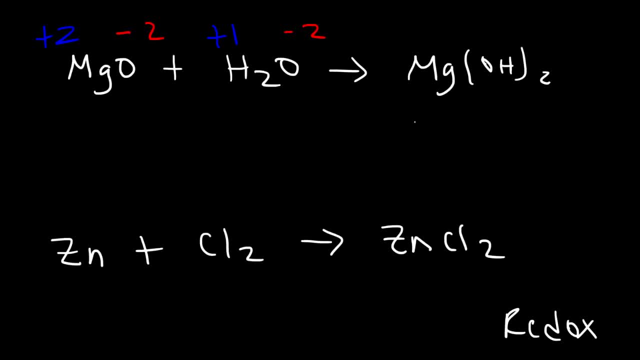 Hydrogen has a positive one charge. Now, magnesium hydroxide is composed of Mg plus two and two hydroxide ions, But, as you can see, magnesium still has an oxidation state of positive two. Now let's focus on hydroxide. 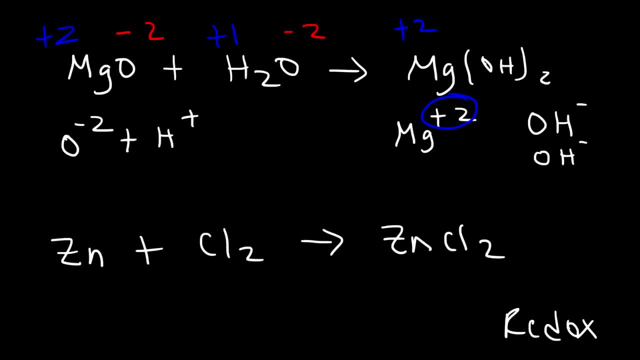 Hydroxide is oxide plus hydrogen. If you want to solve it, You know that hydrogen is going to be a redox reaction. It's going to have a positive one charge And oxygen is going to have a negative two charge. When you add up negative two and one, you're going to get the net charge of a hydroxide. 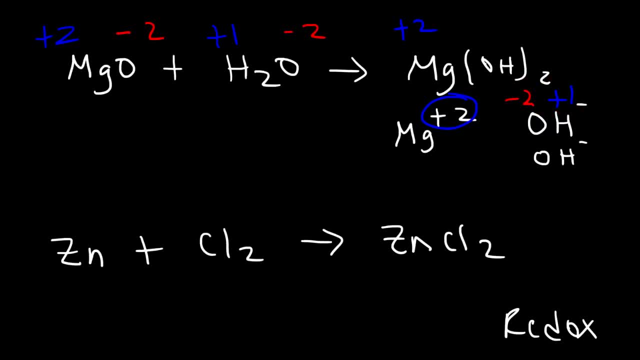 ion, which is negative one. So in magnesium, hydroxide oxygen is still negative two and hydrogen is plus one. So notice that the oxidation state of magnesium did not change: It's still positive two. The oxidation state of hydrogen is still the same. 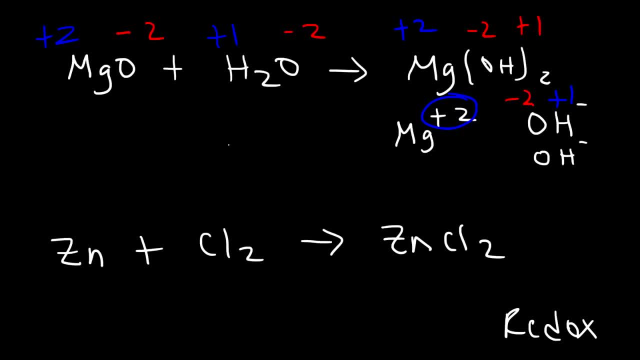 It's positive one And the oxidation state of oxygen has not changed. If the oxidation state does not change, that means there was no transfer of electrons And so this is not a redox reaction. Now let's analyze the second example: Zinc and chlorine has an oxidation state of zero. 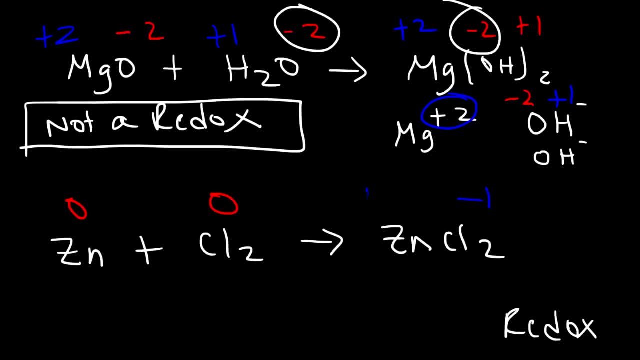 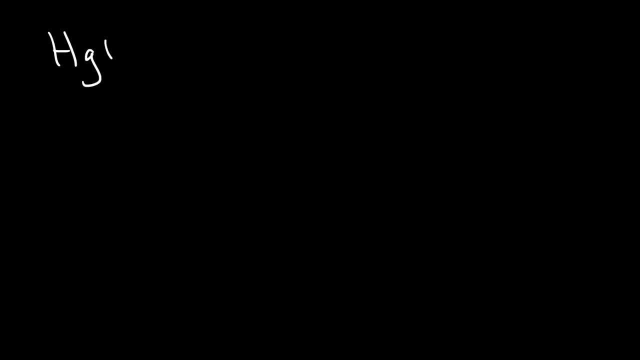 In zinc, chloride Chlorine has a negative one oxidation state. Zinc has a positive two oxidation state. So notice that zinc is being oxidized. Therefore there's a transfer of electrons which makes this reaction a redox reaction. Now consider these two decomposition reactions. 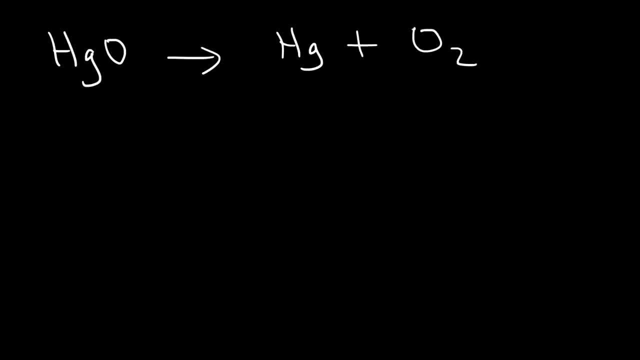 When mercury oxide is heated, it decomposes into mercury and oxygen gas. And if you were to heat calcium carbonate, it will decompose into calcium oxide plus carbon dioxide. So which of these decomposition reactions is a redox reaction? Looking at the first example, we have oxygen as a pure element on the right side. 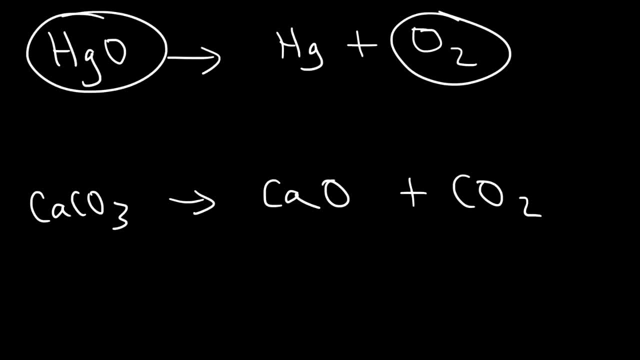 And then that same element is within a compound. So the second example- I mean the first example- is a redox reaction. In the second example there are no pure elements. All we have are just compounds. So the second example is not a redox reaction. 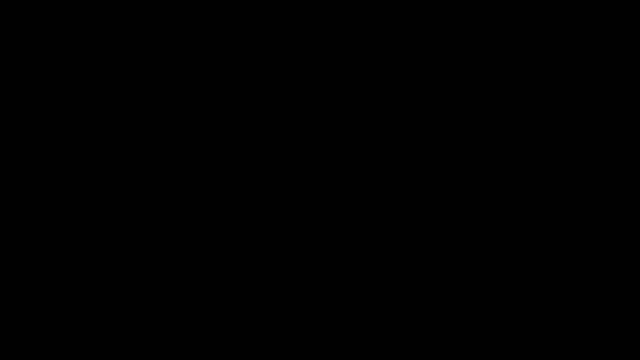 That's a quick way to tell. So now I'm going to give you a list of reactions and determine which ones are redox and which ones are not. So feel free to pause the video if you want to. So the first example: is it a redox reaction? 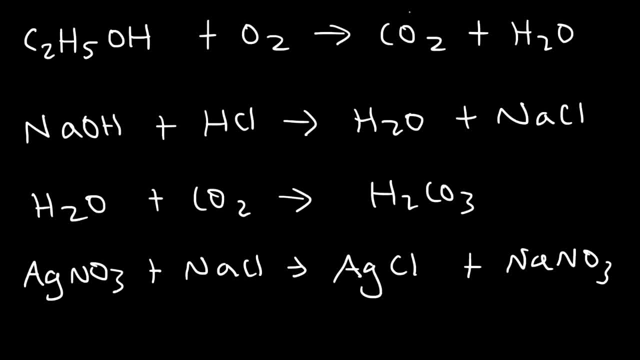 Combustion reactions are always redox reactions. So the first example is it a redox reaction? Combustion reactions are always redox reactions. Here we have a pure element on one side and then that same element is inside a compound. 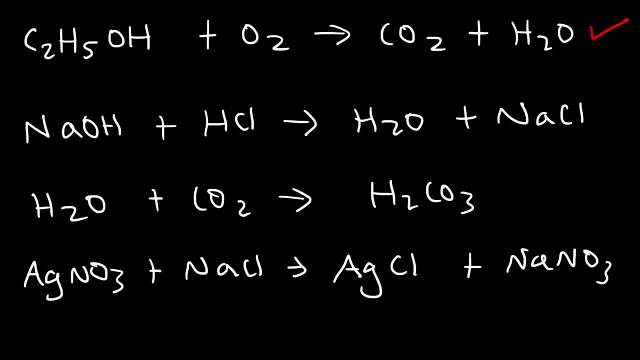 So the first example is a redox reaction. What about the second example? Notice that there are no pure elements in this example. So this is not a redox reaction. Acid-based neutralization reactions are not redox. Any time you have a double replacement reaction, it's never going to be a redox reaction. 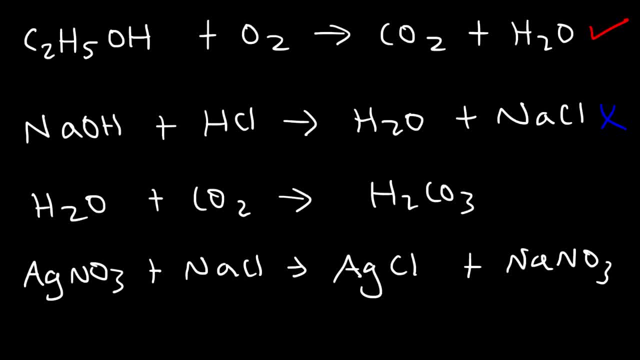 But all single replacement reactions will be a redox reaction. The third example is a combination reaction and there are no pure elements, So therefore this is not going to be a redox reaction. The last one is a double replacement reaction, specifically a precipitation reaction. 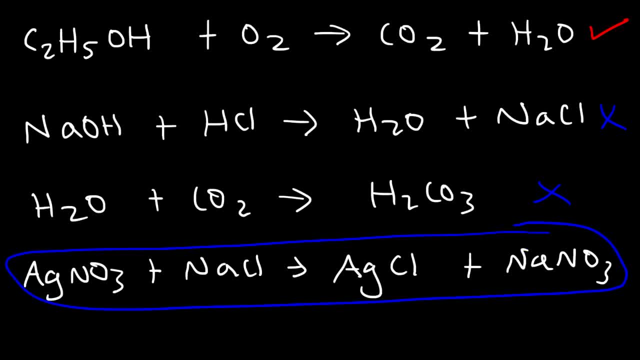 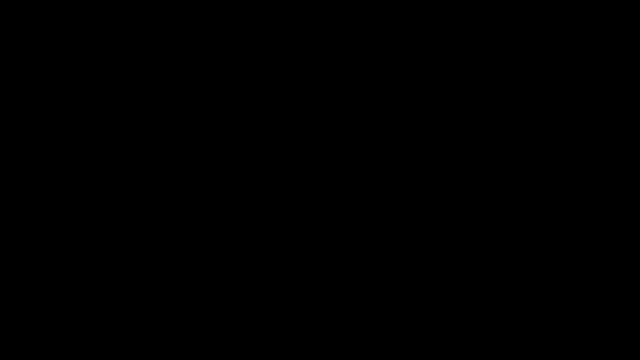 And, as we can see, all we have are just four compounds in this reaction. There are no pure elements, so it's not a redox reaction. So, to review, all combustion reactions are redox reactions. Redox reaction, Redox reaction.